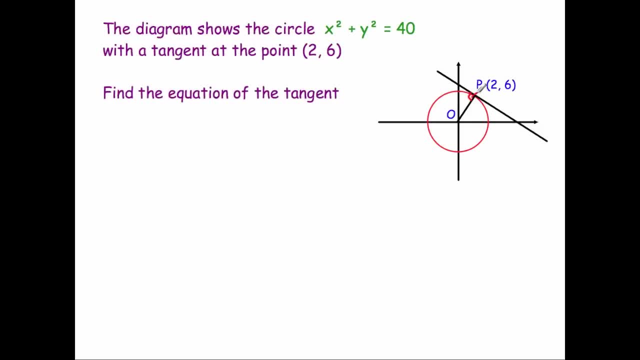 that these two will meet in 90 degrees. So, in other words, you know that this line is perpendicular to this line. So what we're going to do is, first of all, we're going to find the gradient of OP. okay, So the gradient of OP, of OP. Now, the gradient is equal to: 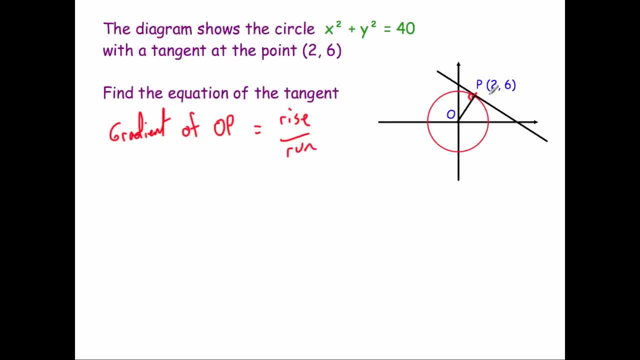 rise over run. okay, Now the rise here. well, it goes across two, so the run's two and the rise it goes up. six is six. okay, If you divide the rise by the run, six divided by two will give you three. So the gradient of OP is equal to three. Now the gradient. 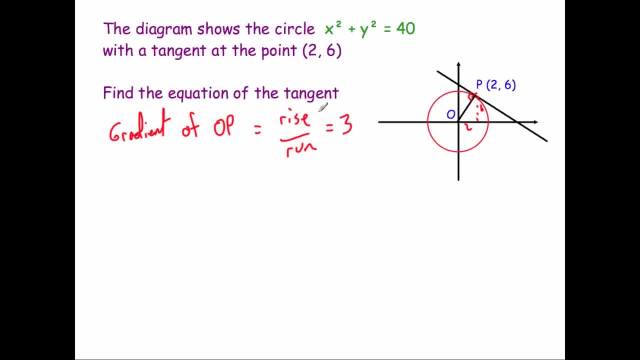 of the tangent then, because it's perpendicular to it, will be the negative reciprocal. So the gradient of the tangent, of the tangent, that's going to be the negative reciprocal of that. So the negative. well, the reciprocal of three is a third Negative reciprocal minus three. 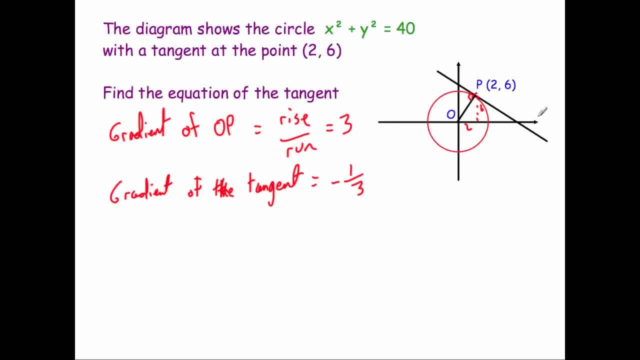 minus one third. So we know this line here has a gradient of minus one third. Now let's find the equation of it. Well, the equation of a straight line is in the format: y equals mx plus c. Now we know this gradient, the m. so it's y equals minus a third, x plus c. 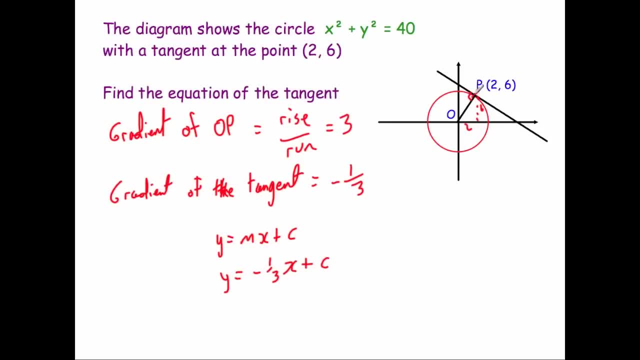 Now also, we know a point on the line, We know the point p is on the line and that point p is the point two six. So if we put these in here we can get the c and then know the equation of the tangent. 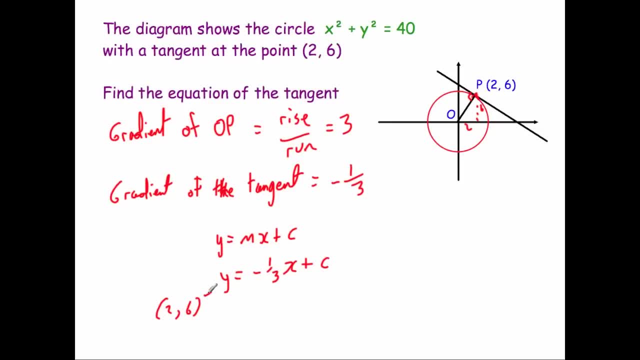 So let's put the point in here. So let's put in two, six into here, So y. well, the coordinate comes in the format xy, so we're going to get six equals minus a third times x. Now x is equal to two, so times two. 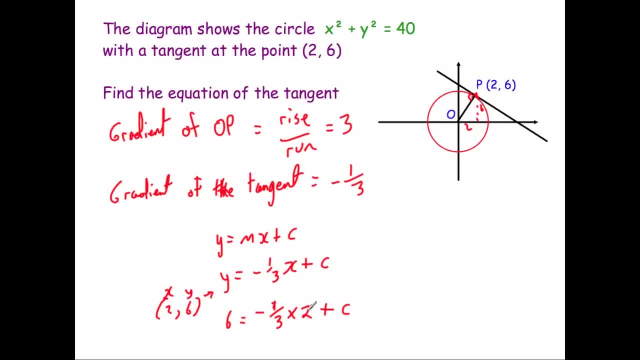 plus c. Well, let's work out our minus a third times two. Well, minus a third times two is minus two thirds. so we're going to get six equals minus two thirds plus c. And we were trying to find out what the c is. so we need to get rid of this minus two thirds. So we're 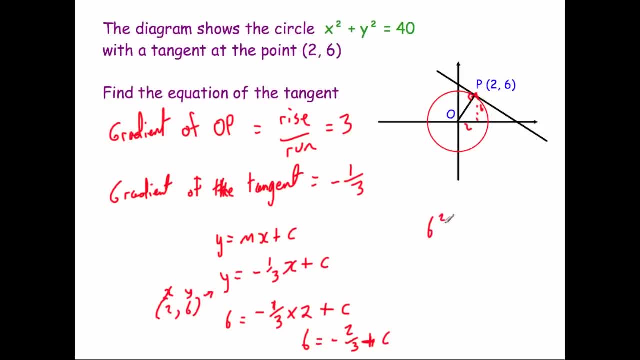 going to add two thirds to both sides, So that would give us that six and two thirds equals c. We can make this a top-heavy fraction if we wanted to, so we could do: six times three is equal to 18, plus two is 20, so that's. 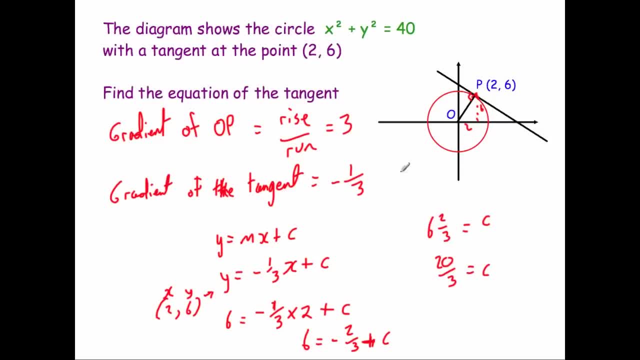 20 over three equals c. Either one's fine. Now we want to find the equation of the tangent. so that's going to be: it's y equals mx plus c. We know the gradient's equal to minus one third. so it's y equals minus one third x.